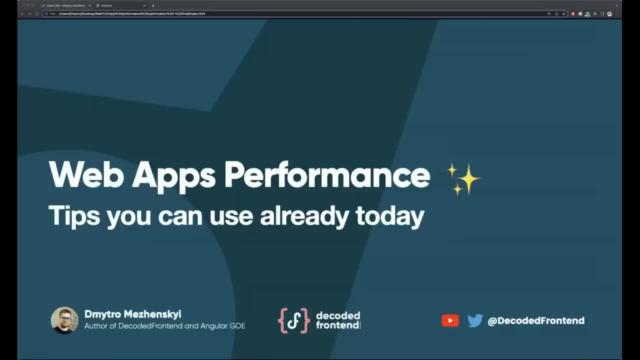 And I'm also the author of YouTube uh channel, Decoded Frontend, as it was already mentioned. Um, there I focus on uh mostly advanced Angular topics and my videos mostly about that. So if you work with this uh framework- with Angular framework, I mean- then please can go subscribe. 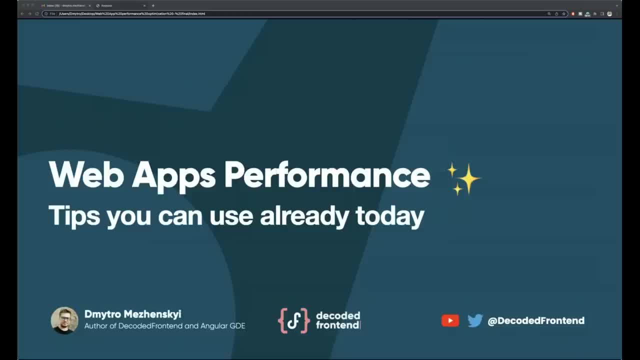 to the channel. I'm pretty sure that you will find a lot of interesting stuff there. But today I would like to talk with you about uh topic that is not strictly related to Angular and uh. it is more, you know, a generic one, um, that fits any frontend frameworks like React. 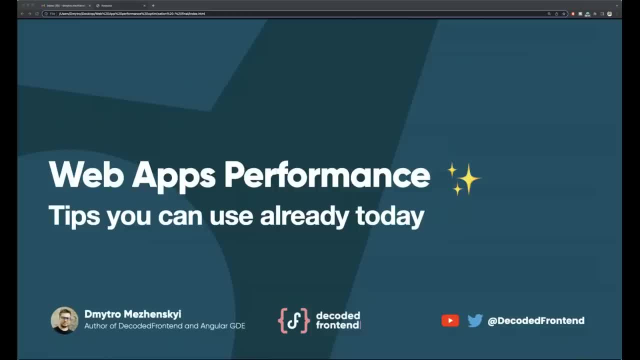 ViewJS or even vanilla JavaScript Project. And, yeah, it will be some set of tips that you can use already now 段, additional setups or anything else, or even if they require some setup. it is quite simple ones, but those tips can give you some performance boost for your. 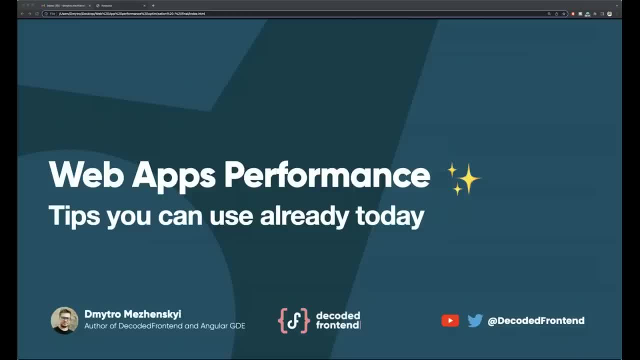 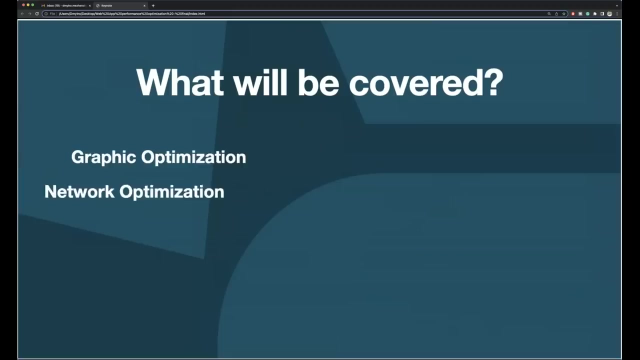 existing and future web applications. there will be tips for, so say, different levels, like for juniors, for more experienced developers. I will try to cover all of them and yeah, alright, then let's get started. and yeah, this is main topics that we will cover. there will be four sections. we will talk about graphic. 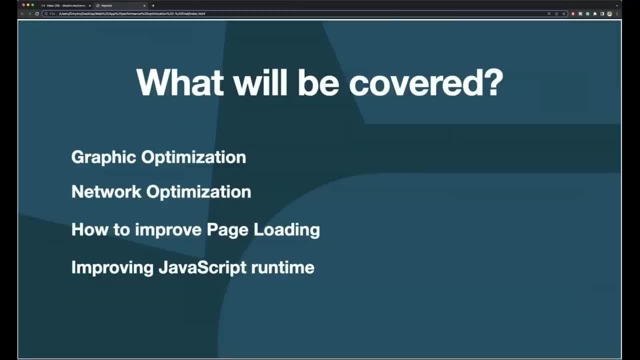 optimization, images and and so on. network optimization: we will talk how to improve page loading and how to improve page loading and how to improve page loading and how to improve JavaScript runtime performance. also, in the end, there will be additional bonus section like team performance, so stay with us if you want to hear that. and, as I said, each of this section: yeah, 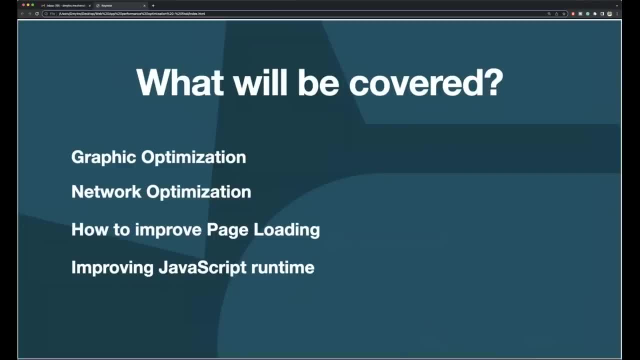 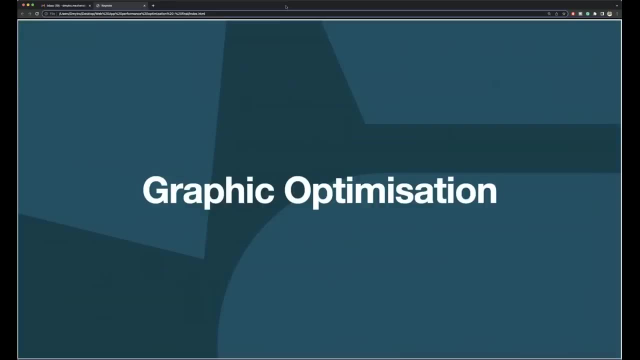 will have some set of small tips and tricks you could apply for your project as well. yeah, and let's get started with the very first topic called graphic optimization. well, unoptimized graphics, it is one of the most, so say, popular causes of bad performance and UX, so that's why you 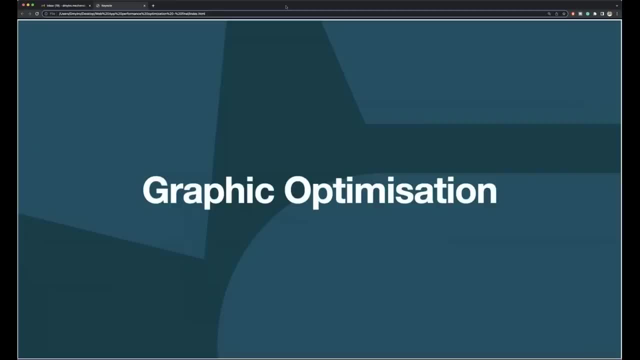 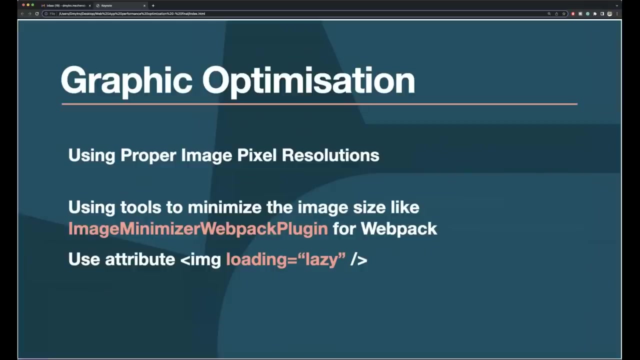 have to pay attention to it in the first place, and it is better to care about that already, from the very beginning, obviously, when you start the project. and yeah, let's have a look what we could make better. so, first of all, and the easiest, is to use proper image pixel resolution for raster images like PNG. 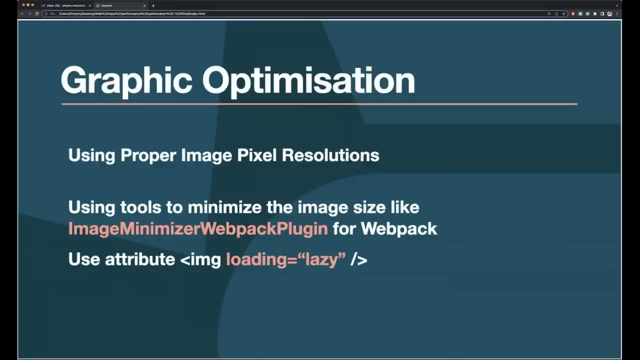